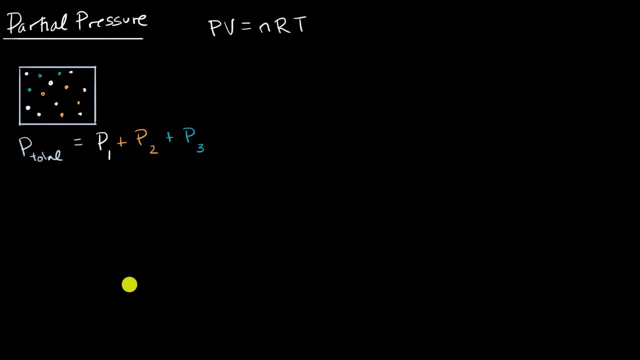 times the ideal gas, constant times the temperature. And so if you were to solve for pressure here, just divide both sides by volume, you'd get. pressure is equal to nr times t over volume, And so we can express both sides of this equation that way. 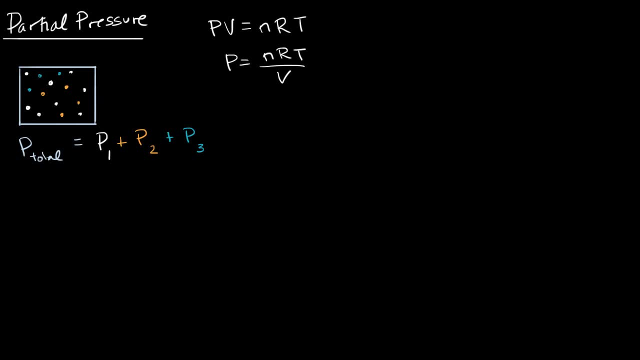 Our total pressure, that would be our total number of moles. so let me write it this way: n total times the ideal gas, constant times, our temperature in Kelvin divided by the volume of our container, and that's going to be equal to. 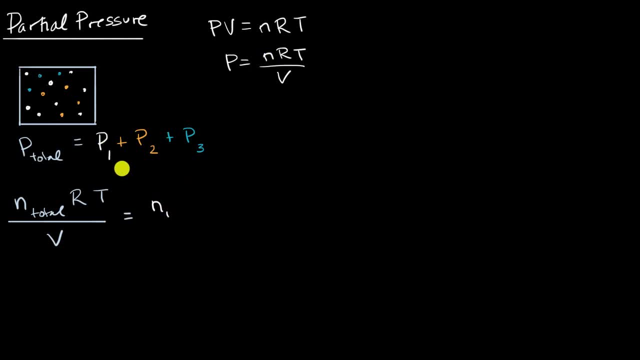 so the pressure due to gas one the number of moles of gas. one times the ideal gas. constant times the temperature. The temperature is not going to be different for each gas. We're assuming they're all in the same environment, divided by the volume. 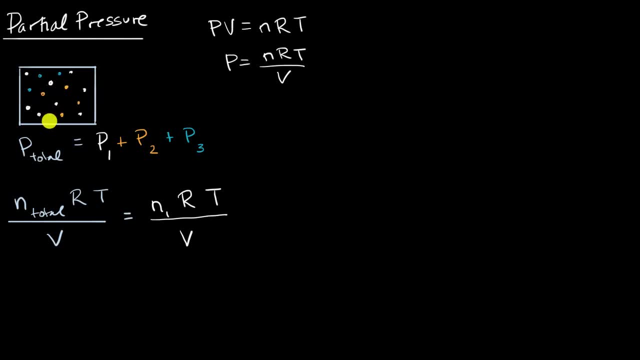 And once again the volume is going to be the same. They're all in the same container in this situation. And then we would add that to the number of moles of gas two times the ideal gas constant, which once again, is going to be the same for all the gases. 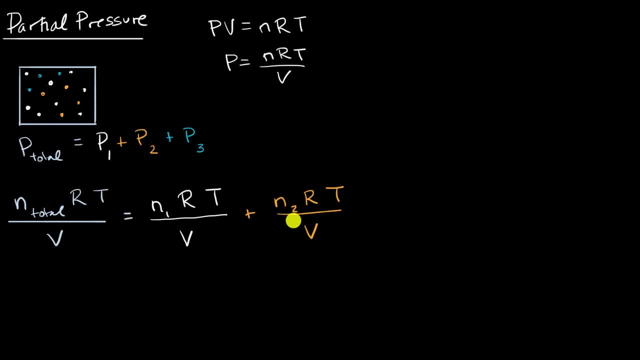 times the temperature divided by the volume, And then to that we could add the number of moles of gas three times the ideal gas constant times the temperature divided by the volume. Now I just happen to have three gases here, but you could clearly keep going. 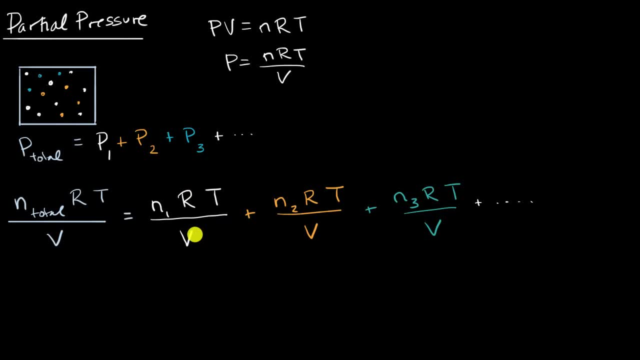 and keep adding more gases into this container. But when you look at it mathematically like this, you can see that the right-hand side, we can factor out the RT over V and if you do that you are going to get n one plus n two. 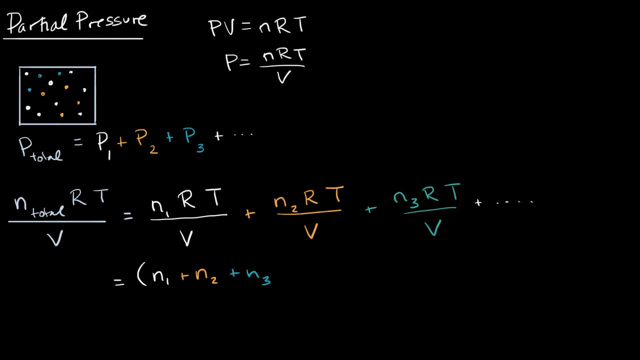 plus n three- let me close those parentheses. times RT, RT over V And this right over here is the exact same thing as our total number of moles, If you say the number of moles of gas one plus the number of moles of gas two. 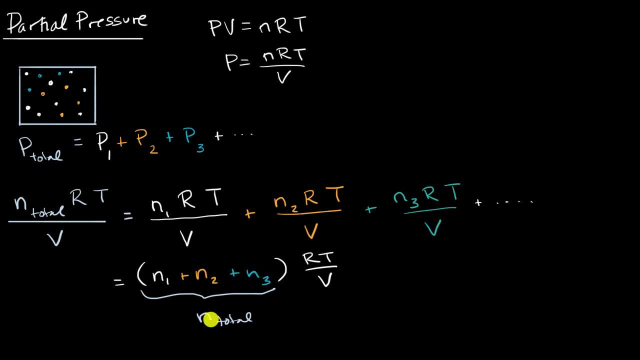 plus the number of moles of gas three, that's going to give you the total number of moles of gas that you have in the container. So this makes sense mathematically and logically And we can use these mathematical ideas to answer other questions. 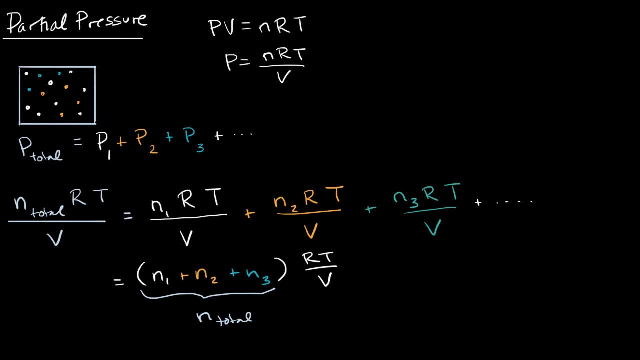 or to come up with other ways of thinking about it. For example, let's say that we knew that the total pressure in our container due to all of the gases is four atmospheres. And let's say we know that the total number of moles 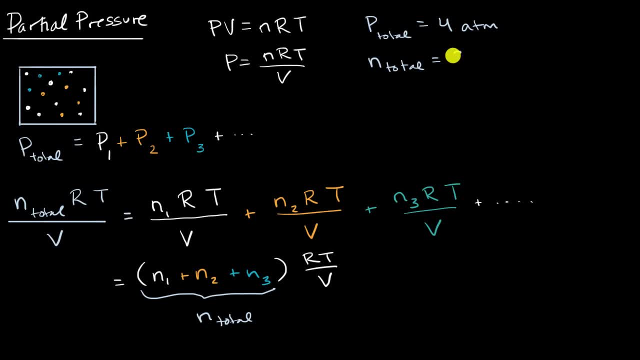 in the container is equal to eight moles. And let's say we know that the number of moles of gas three is equal to two moles. Can we use this information to figure out what is going to be the partial pressure due to gas three? 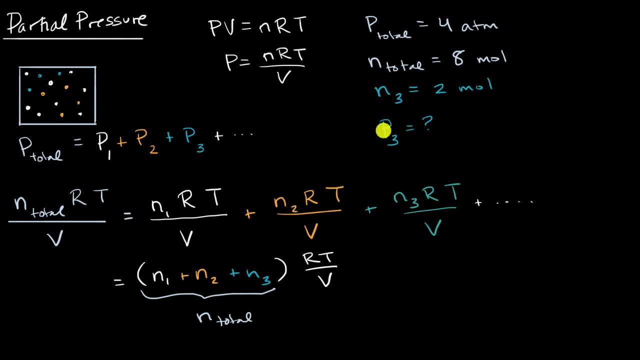 Pause this video and try to think about that. Well, one way you could think about it is the partial pressure due to gas three over the total pressure. over the total pressure is going to be equal to, if we just look at this piece right over here: 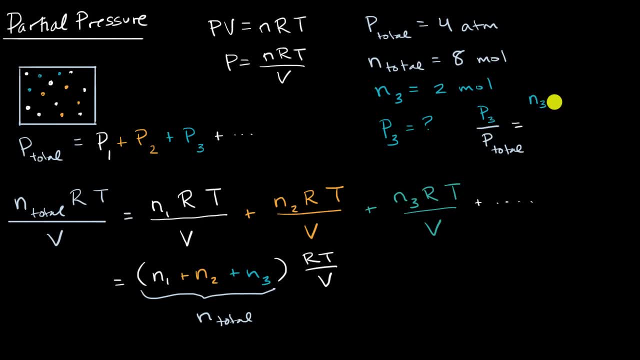 it's going to be this. It's going to be the number of moles of gas three times the ideal gas constant, times the temperature divided by the volume, And then the total pressure. well, that's just going to be this expression. So the total number of moles times the ideal gas constant. 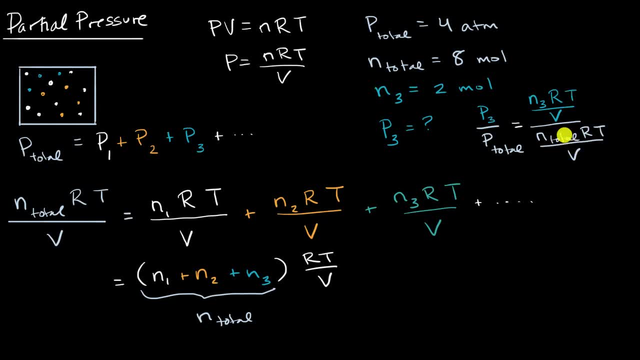 times that same temperature because they're all in the same environment, divided by that same volume. they're in the same container And you can see very clearly that the RT over V is in the numerator and the denominator. So they're going to cancel out. 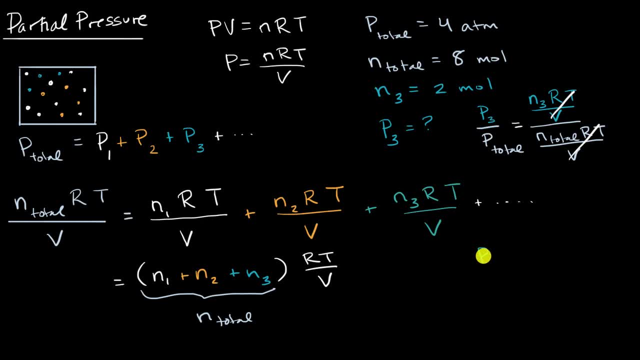 And we get this idea that the I'll write it down here: the partial pressure due to gas three over the total pressure is equal to the number of moles of gas three divided by the total total number of moles. And this quantity right over here this is known as. 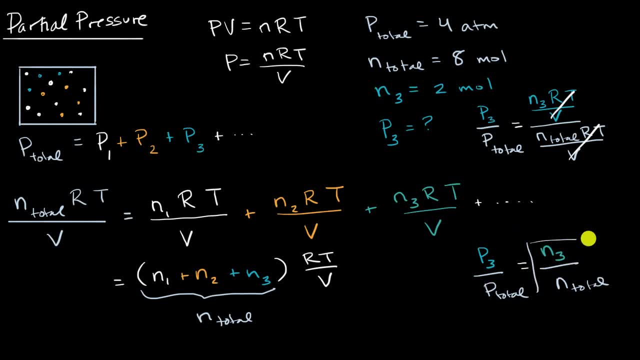 and this quantity right over here. this is known as the mole fraction. Let me just write that down. It's a useful concept And you can see the mole fraction can help you figure out what the partial pressure is going to be. So for this example, if we just substitute the numbers,